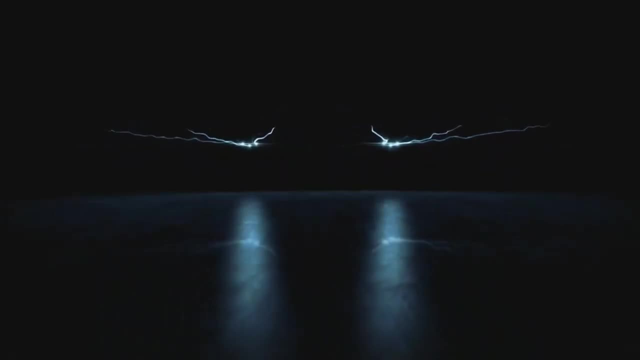 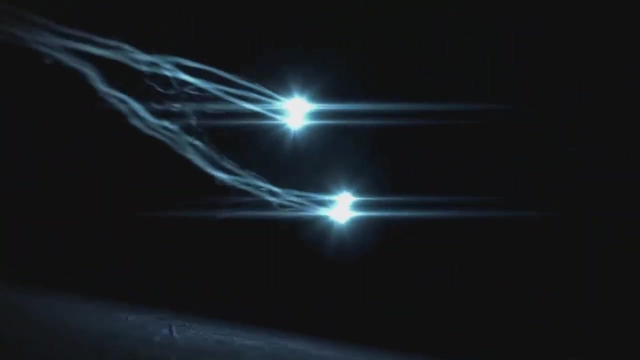 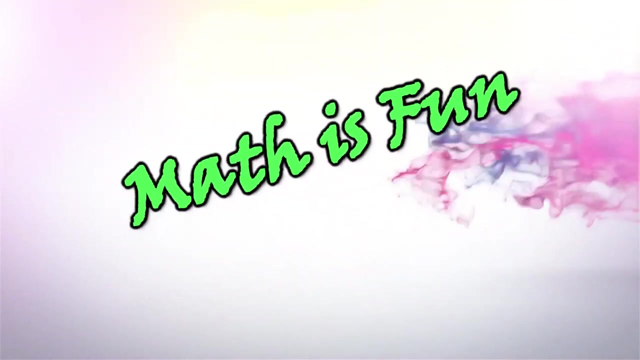 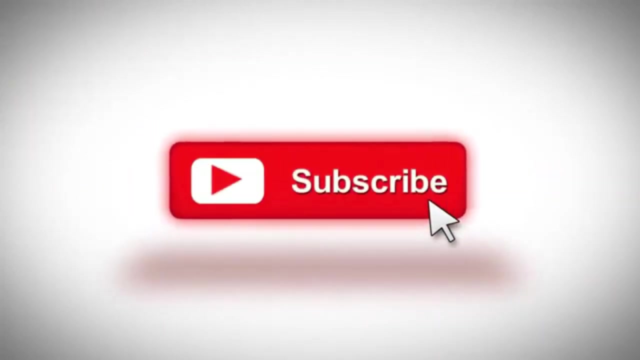 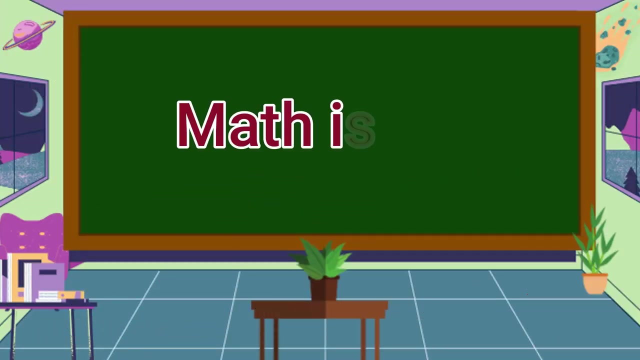 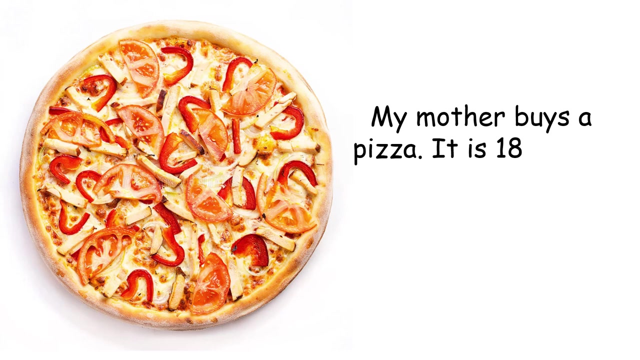 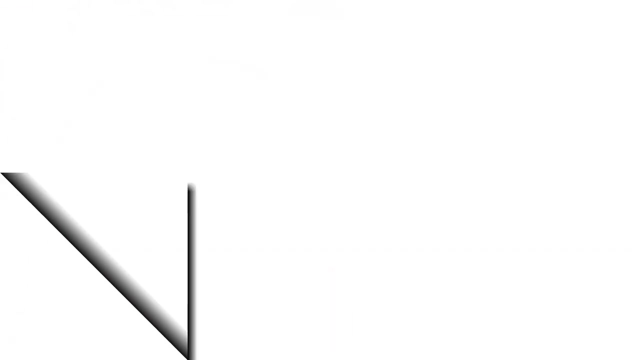 Thank you for watching. Hello everyone, Welcome to. Math is Fun. Our lesson for today is all about visualizing circumference of a circle. My mother buys a pizza. It is 18 inches in diameter. What is the circumference of the pizza? Before we are going to get the circumference of this pizza. 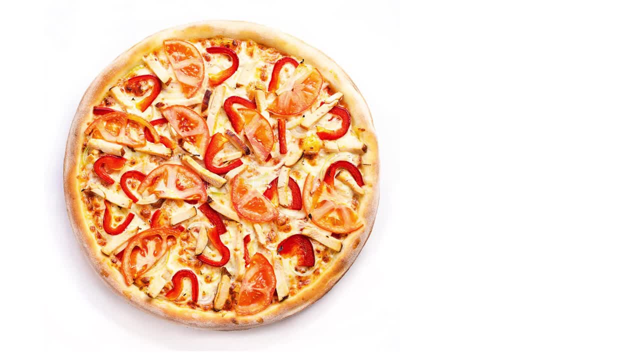 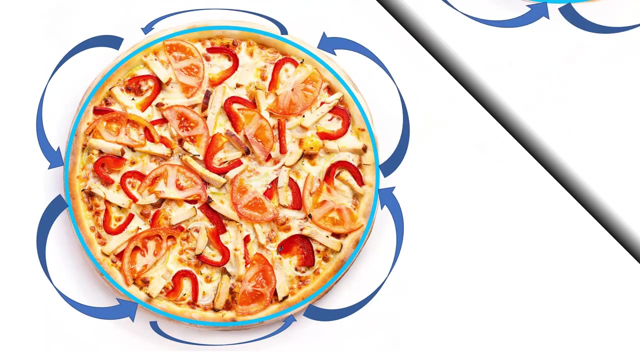 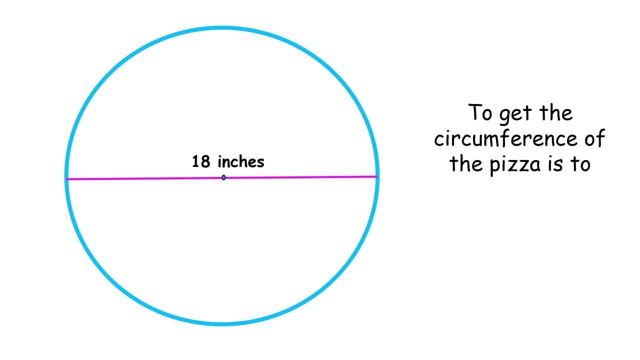 we are going to discuss first what is a circumference? When we say circumference, it is the distance around the circle. This pizza is a round shape, so we are going to get the circumference. One way to get the circumference of the pizza is to measure the distance around it using a tape measure. 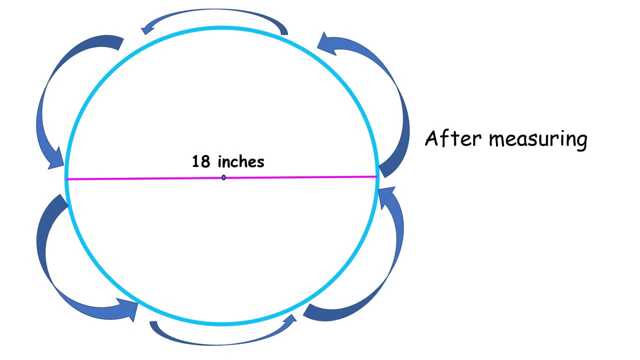 After measuring it, the circumference of the pizza is more than 56 inches, but less than 57 inches. What is the exact circumference of the pizza? Before we are going to answer, we are going to discuss first the ratio between the circumference of the circle to each diameter. 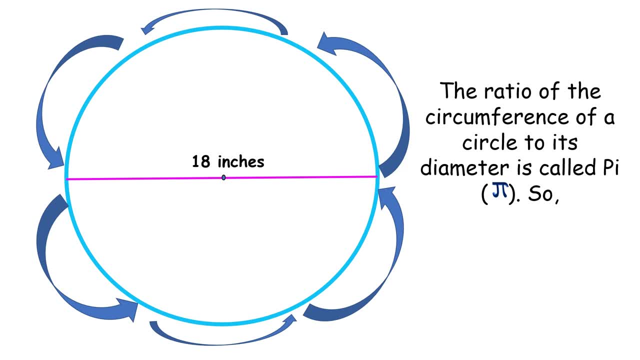 The ratio of the circumference of a circle to each diameter is called pi. This is the symbol for pi, So pi is equal to circumference divided by diameter. The approximate value of pi is 3.14 or 22 over 7.. From the concept description: